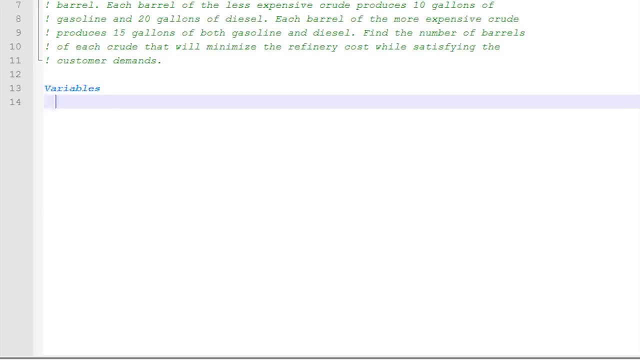 I'm going to make those integer variables as well. So let's go ahead and program this in the AP monitor modeling language, and I'm going to have x greater than 0 and y is greater than 0.. Now I have my equations as well. 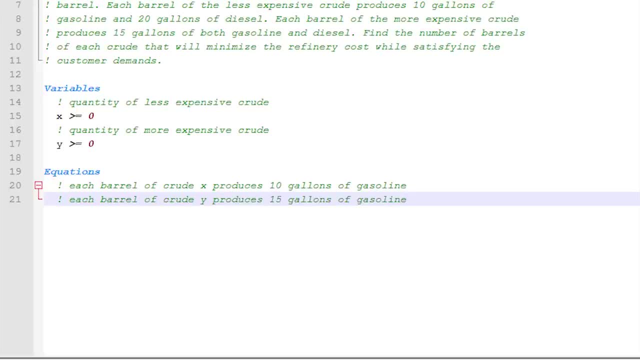 These are the. the first one is the gasoline constraint equation, So the first type of crude can produce 10, and the second can produce 15,. that has to be greater than or equal to 100. And then the diesel constraint as well. 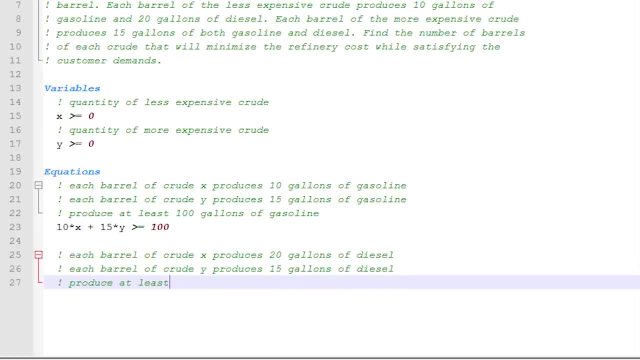 So I have, in this case, 20 times x plus 15 times y, greater than or equal to 160.. Okay, now I want to minimize the total cost. I have my cost of each crude and I come up with my objective function here. 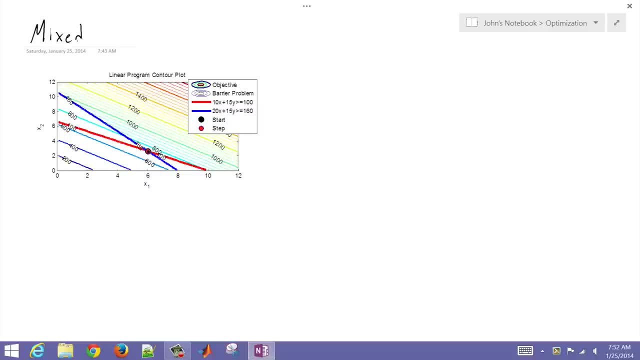 which is 80 times x and 95 times y. This is our mixed integer linear programming problem and there is our optimal solution There at x equals 6 and y equals 2.67,. I also named those x1 and x2.. 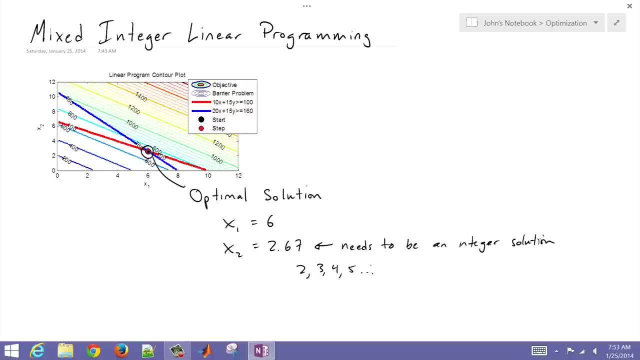 Okay, so don't be confused by that. So I want integer values for those 1,, 2,, 3,, 4,, 5, 6.. And I'm going to do a branch and bound technique or an outer approximation technique. 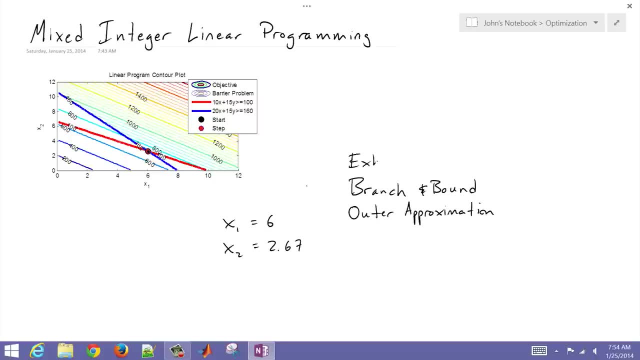 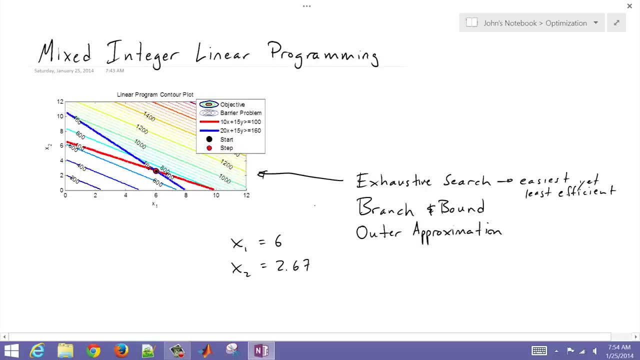 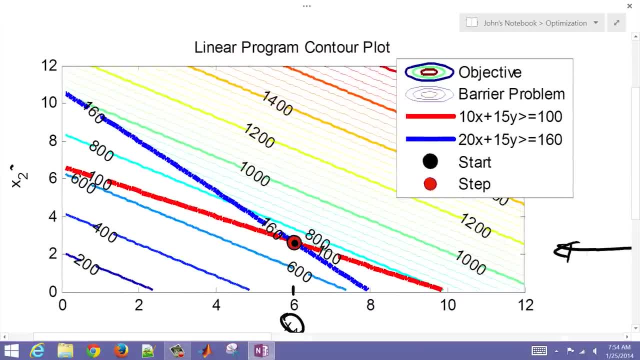 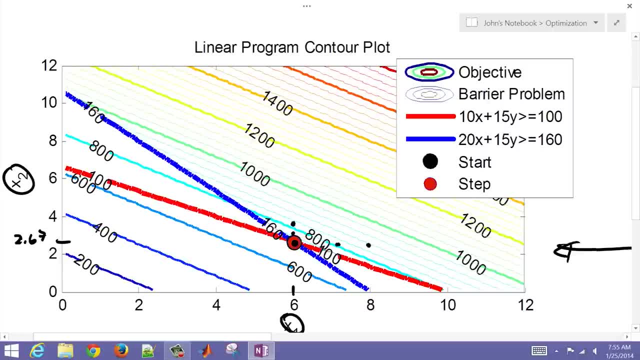 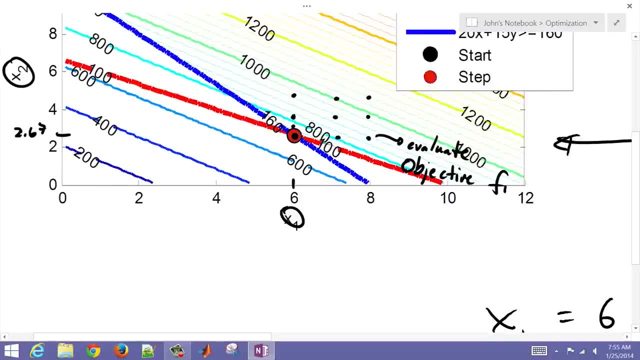 where I have potential integer solutions. So I can't buy a partial of a barrel, I have to buy a full barrel. So I'm going to evaluate the objective function at every possible solution and I also know that I have non-feasible solutions. 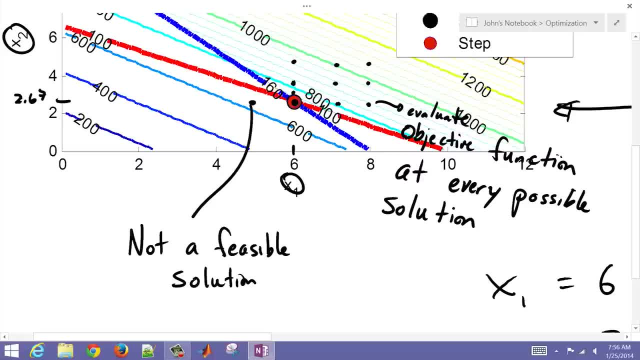 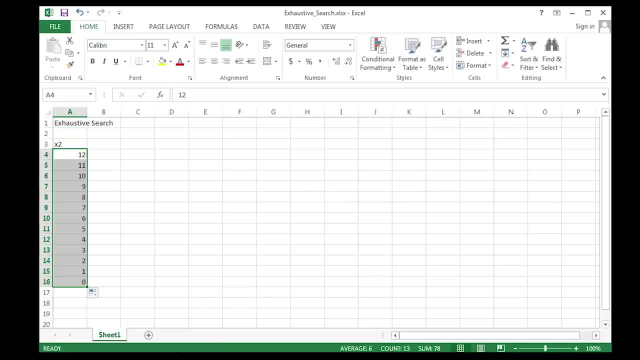 or infeasible solutions at certain points. So let me go over to Excel for this. I'm going to first of all. I'm going to go over to Excel. First of all. I'll do my X2, I'll also use Y and then just go ahead and create that plot. 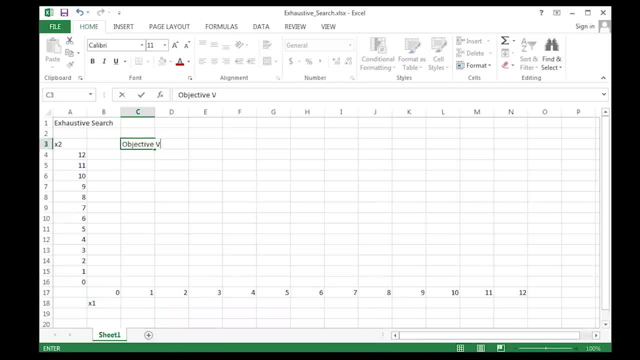 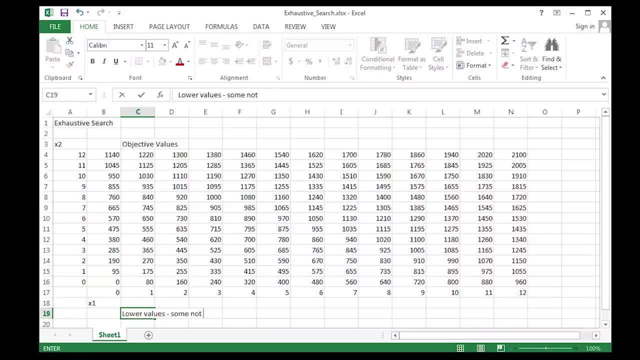 These are my objective values. I'm going to just get my objective function here and let me go ahead, and okay, so now I can see my objective function values for different options of you know, X and Y. Now I also have lower values. 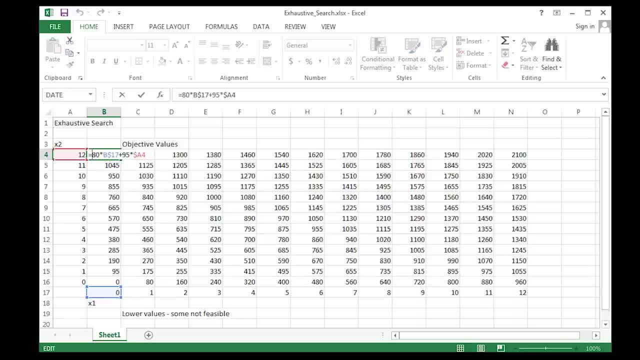 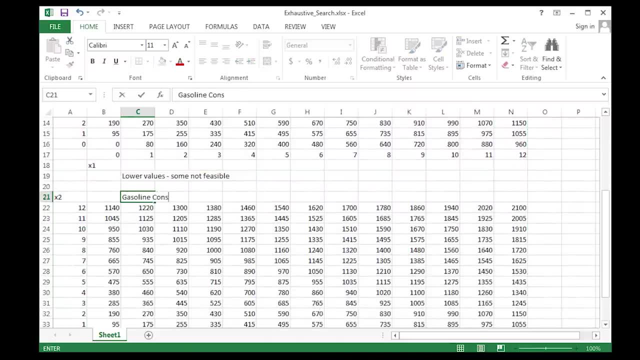 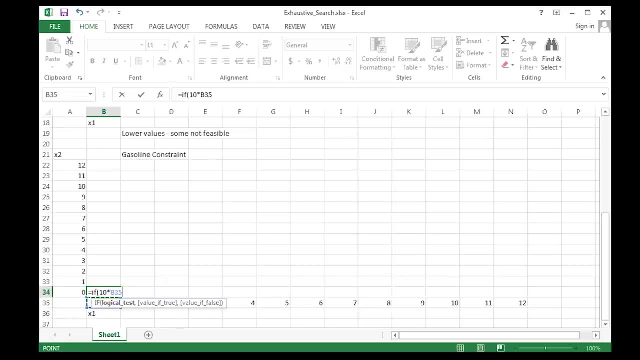 Some of them are not feasible. okay, so some of these are not feasible because I need to have a certain amount that I need to produce of each. Okay, so let me go in here and I'm going to make sure that it's less than. 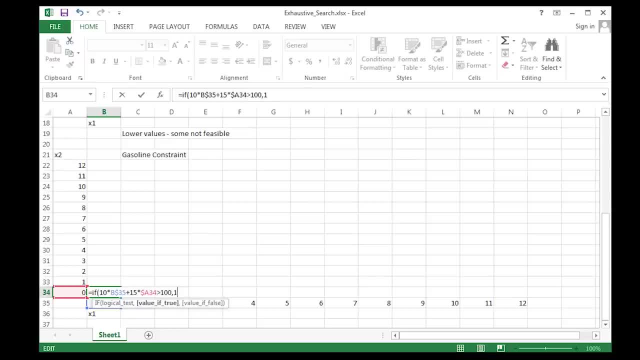 or greater than or equal to or greater than 100.. I'm just going to do greater than 100 first and I'll show you how that changes with greater than or equal to 100.. There you can see. ones are the ones that are feasible. 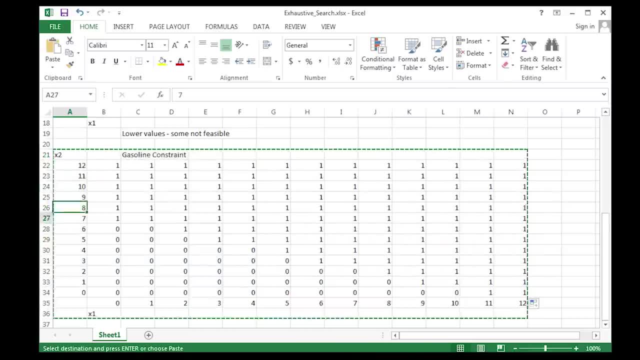 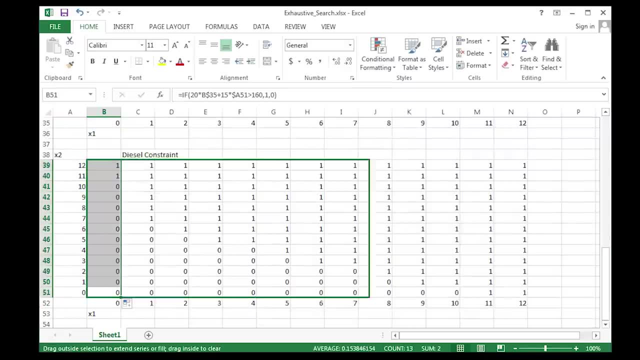 I'm also going to do the diesel constraint as well here. Okay, so now the diesel constraint, and that's the ones, are the possible solutions. So what I'm going to do is just multiply by the diesel and the gasoline constraints, and anywhere that's zero is going to be infeasible. 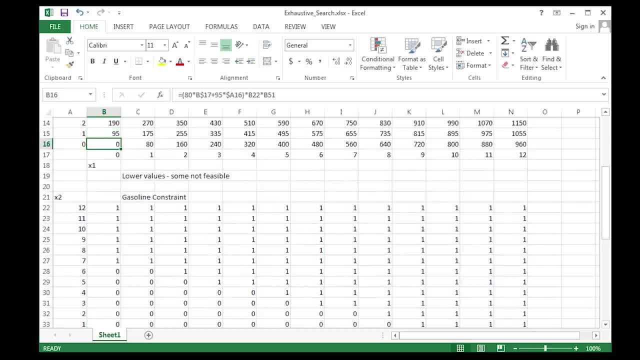 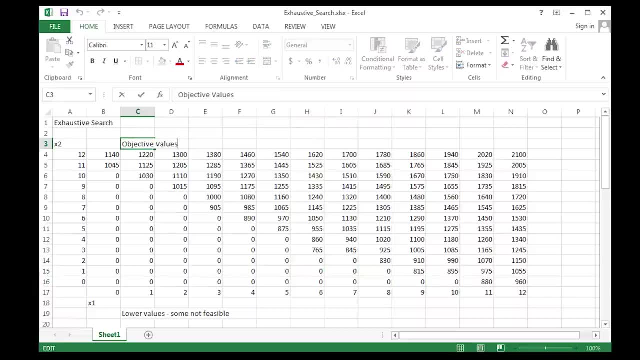 and anywhere that's non-zero is going to be a feasible solution. So this is an exhaustive search. I'm looking over all. let's see all of the potential values. So 13 times 13 values. I have to evaluate those and there's my lowest objective function. 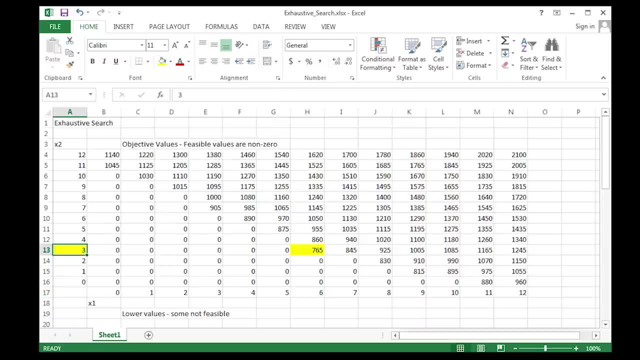 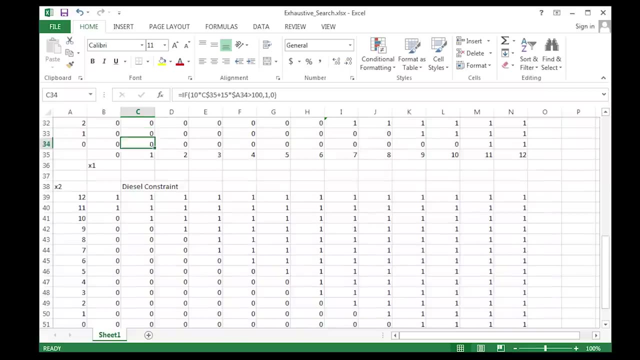 Now, one of the things you'll notice with this is that I did greater than 100.. So let's say I do greater than or equal to 100, and let me go back into the constraints here and I'm going to go ahead and evaluate greater than or equal to 100 instead. okay, 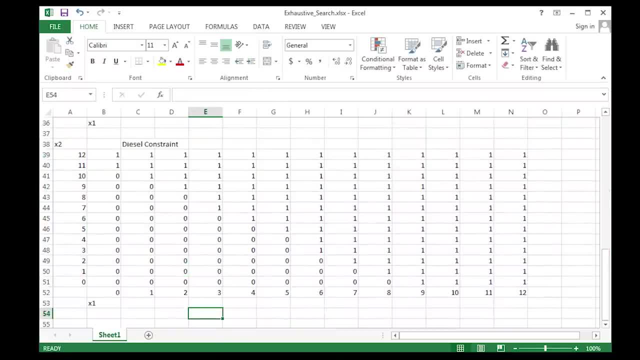 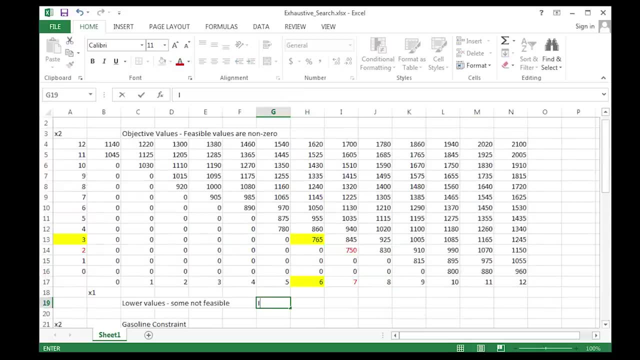 and greater than or equal to 160 for the diesel constraint. And now you can see that I have a different optimal solution because I had an inequality constraint that is greater than versus greater than or equal to. So that's just one thing you have to watch out for in integer programming. 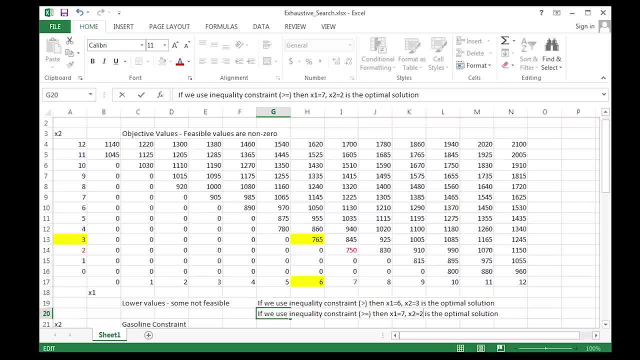 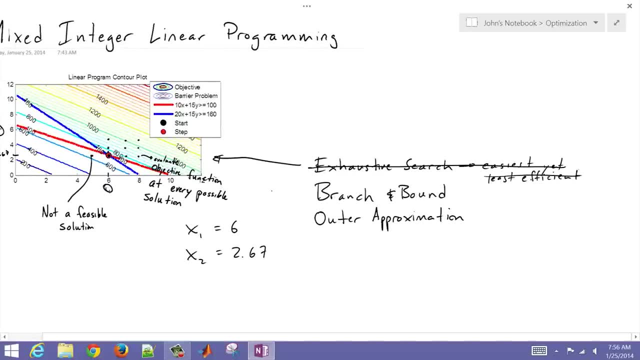 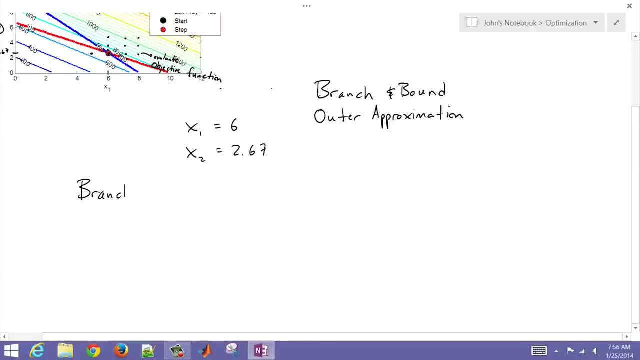 that you have the correct inequality constraints. Okay, so those are my two solutions. That was an exhaustive search. However, that's least efficient. Most people don't use an exhaustive search, except for very simple problems. I'm also going to cover branch and bound now and how to perform that. 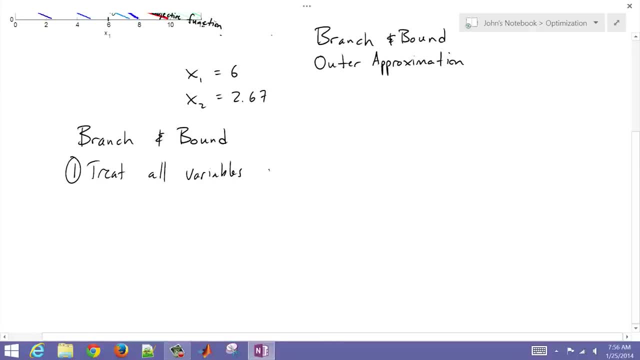 First, you treat all variables as continuous and solve the relaxed problem. This is called a relaxed problem. There's my solution. And then you select one of the variables that's non-integer for branching. Okay, so what we want to do is, you know, select a variable. 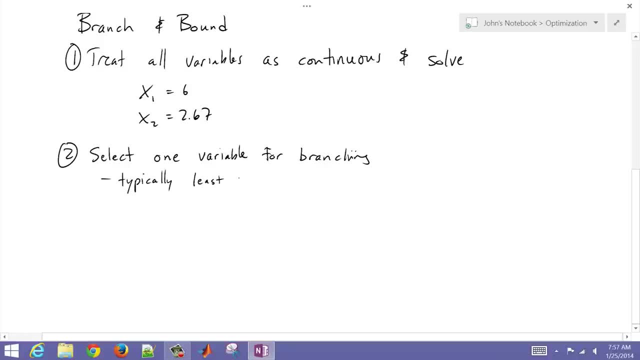 Typically, we select the one that's the least closest to integer value. Okay, so something that's like closest to .5.. Okay, so what we want to do in this case is do the x2 or y value Okay, And what I want to do is do the x2 or y value. 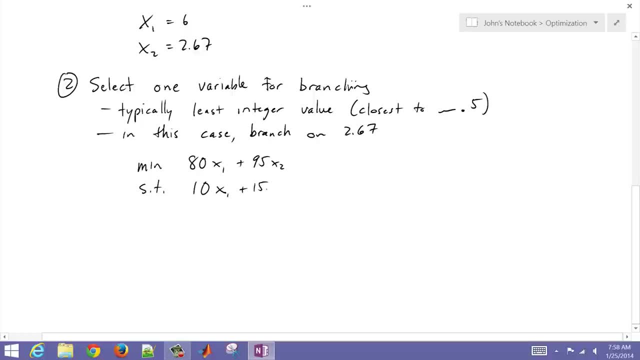 Okay. Okay, we'll do, is you know? just add an extra constraint here to my original problem that X 2 is going to be greater than or equal to 3, and then also less than or equal to 2, and then we will solve. you know, this top part will always solve. 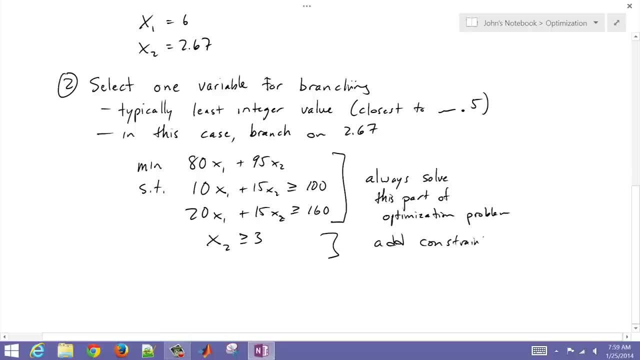 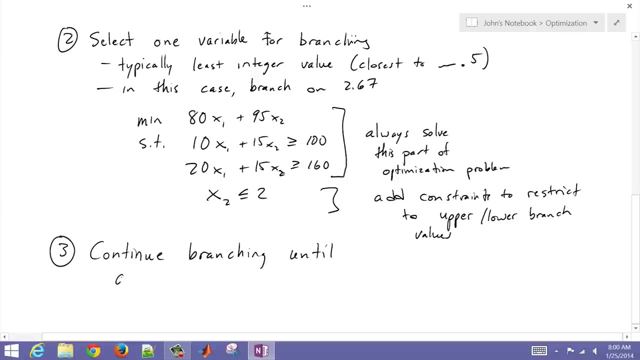 that same part and then add these constraints to restrict the values and and do this branching. okay, the upper and lower values, okay, so we'll do both of those. and then the third is: we'll just continue branching until all of the values are within a certain tolerance of an integer value. okay, all of them are. 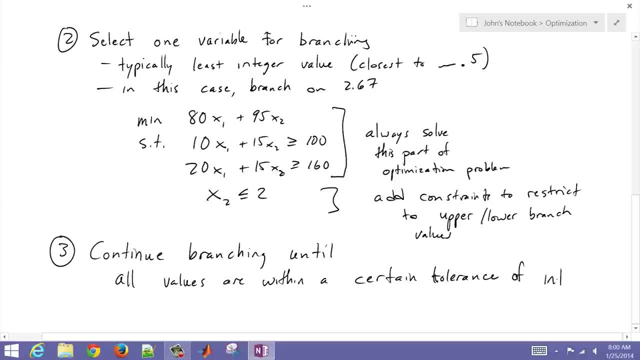 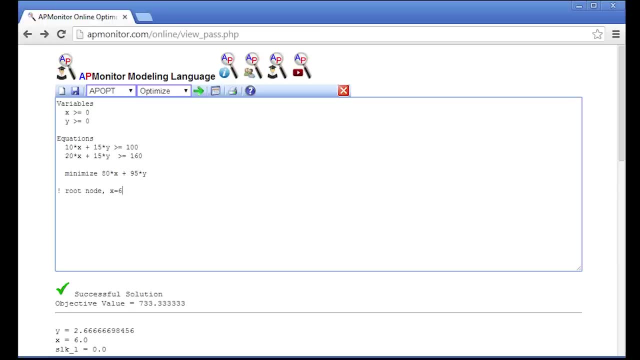 integer values and we don't have any others that we can explore that might be potential solutions. okay, so in this case I'm going to start off with just my relaxed solution. this is my root node and I'm just going to record the solution and the objective function. that's going to be a lower bound for my 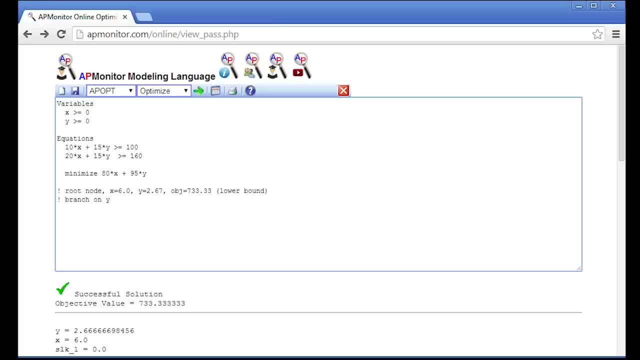 objective function. now I'm going to branch on Y. okay, so Y less than or equal to 3, and then I'm going to add a new constraint to this, one that's going to be less than or equal to 2 and greater than or equal to 3, and go. 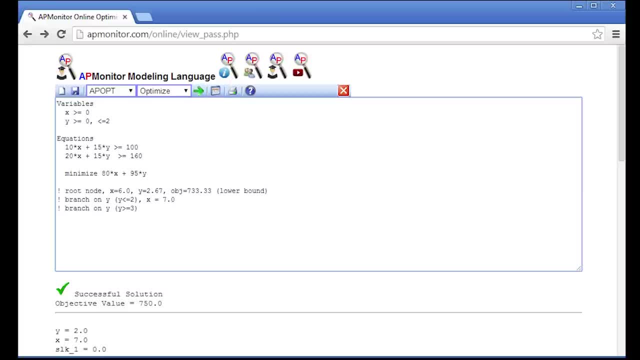 ahead and solve it again. record the solution. so the less than or equal to 2 gave me a solution of my objective function and an upper bound is an integer solution. so it's going to be an upper bound for my objective and I'm going to solve that with greater than or equal to 3 as well, and that's not an 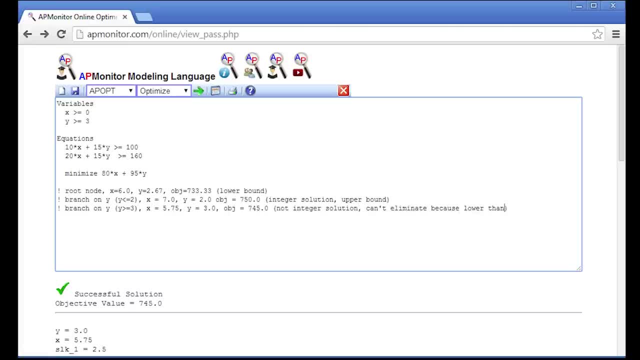 integer solution, but we can't eliminate because it's not. it's lower than the upper bound. okay, so I'm going to branch on X now because that's non-integer, and let me go ahead and do the X branch and then solve the first one. okay, so I 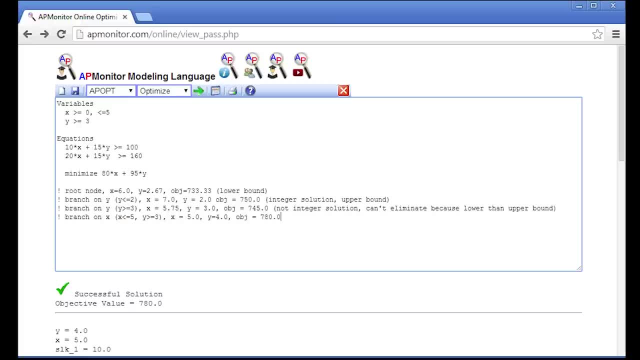 have another integer solution, but not as good as the prior integer solution. okay, now I'm going to do the other branch as well, on X. okay, just putting in those constraints, and I came up with another one integer solution, but not quite as good as the prior one. okay, so no more branches to explore. we'll go ahead and 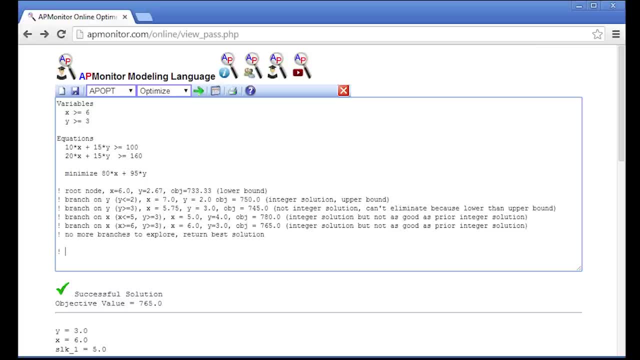 return the best integer solution in this case and that will be our optimal value. Okay, now another way to do this is just put int in front of your variable names and that will enforce them so that they are integer values, and you'll see that it'll come up with an integer solution for you, and you can see some of the 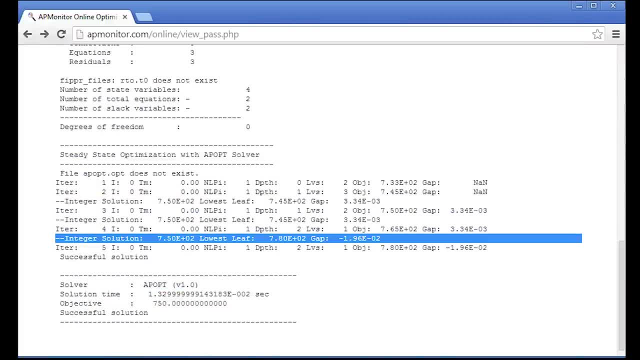 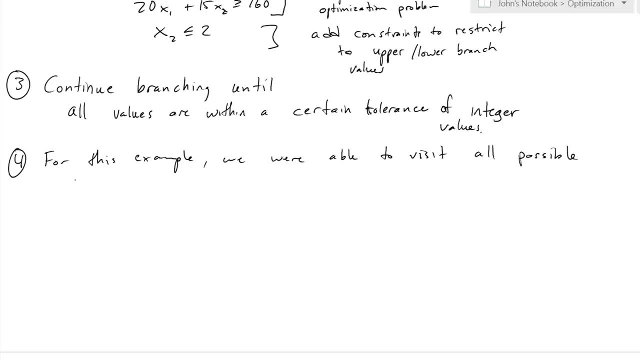 branching. that it does with the solver. Okay, so if you don't want to have to do that yourself, you can solve it like that. For this example, we were able to visit all possible integer points had an objective function less than the upper bound Other cases. it's not possible to visit all the points without excessive. 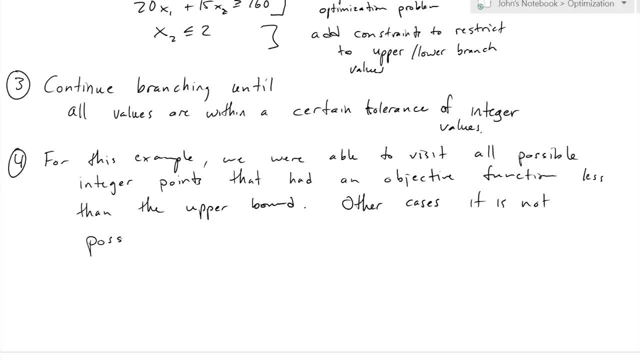 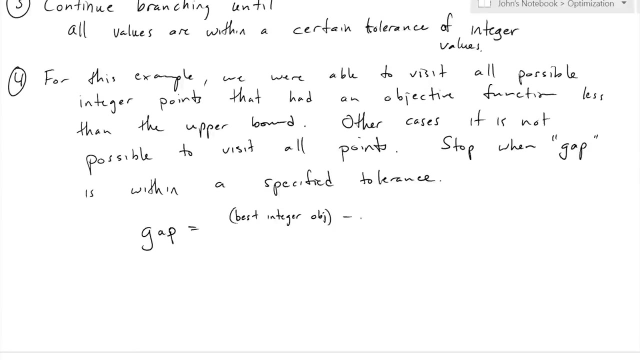 computational time. So typically we stop when we're within a gap of the the best solution possible. So we define gap as the difference between the best integer objective and the lower bound of the relaxed solutions divided by those two quantities added together. As long as we're within a certain tolerance and we 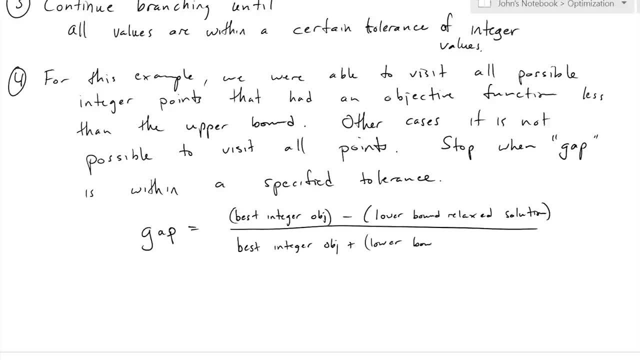 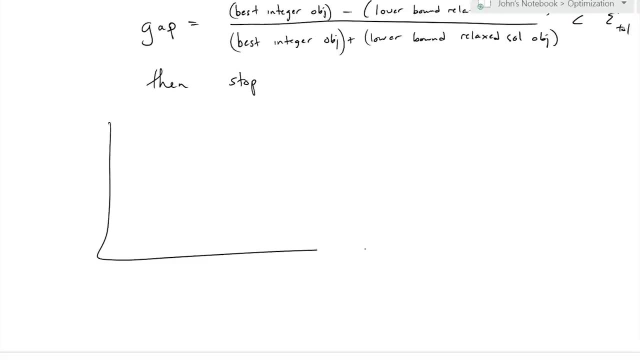 say that we can terminate the, the optimization and accept the best solution. Okay, so let me just graphically depict this. So we have iterations or solutions. Now these are relaxed solutions with bounds, extra bounds, placed on them, and so we might have a root node, for example, that we solved when we removed all. 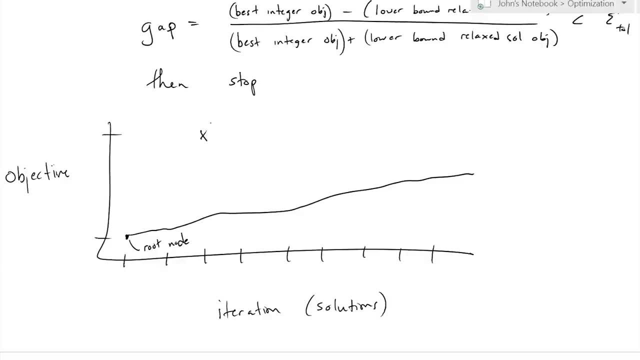 integrality constraints, and then we may have integer solutions along the way that are upper bounds, and then, when we're within a certain gap of the best solution, so we know that that's the lower bound and upper bound, and we stop and say that the best integer solution is our solution to. 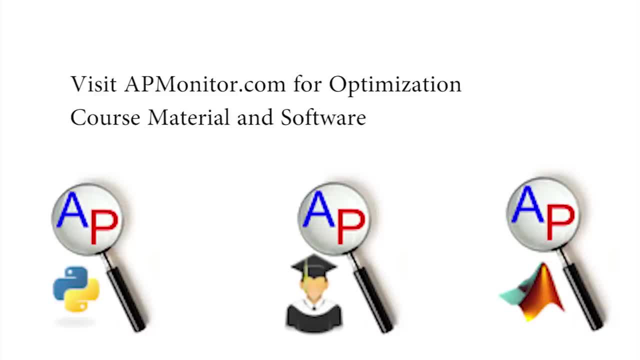 this problem. Visit apmonitorcom for additional course material and optimization software. 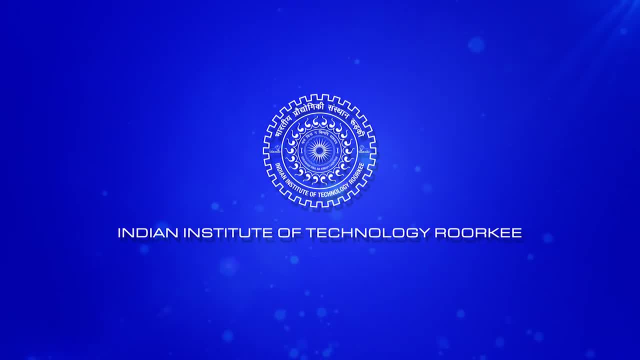 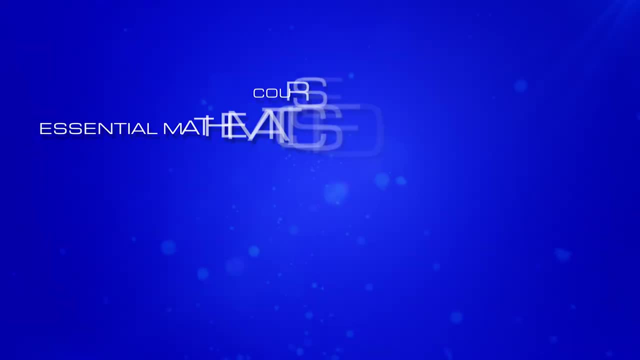 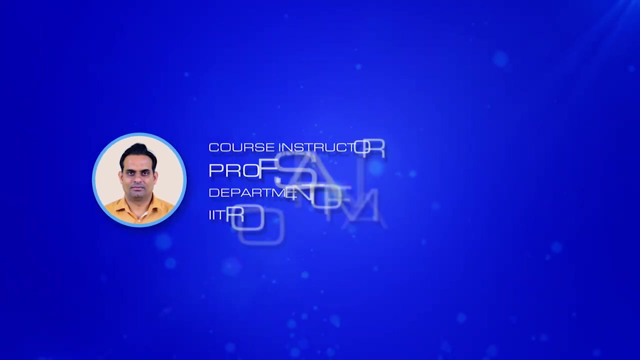 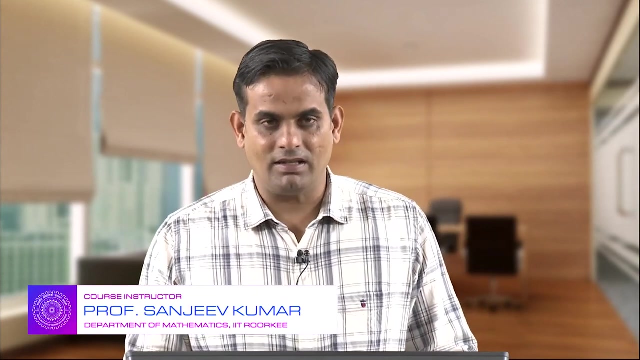 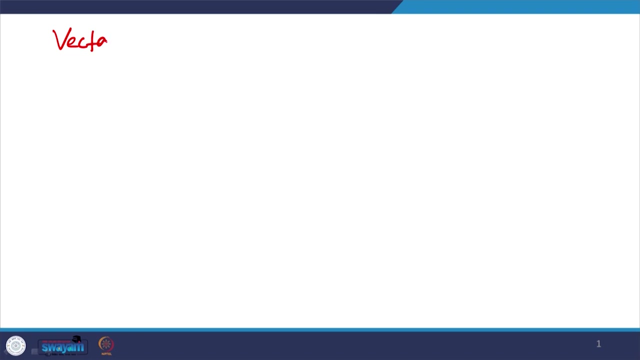 So we start this lecture with the definition of vector spaces. So let us define vector space, So a vector space, V over the field R. So here V is the set of vectors and R is a field of scalars. In general we can define vector space over any arbitrary field, but in machine learning, 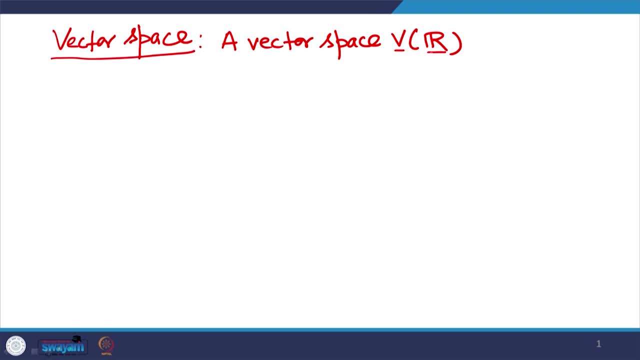 we usually have vectors. those are defined over the field of real numbers. So in this course we will focus on the vectors, or vector spaces. those are defined over the field of real number. So vector space. V- R over a field, R, So a vector space.